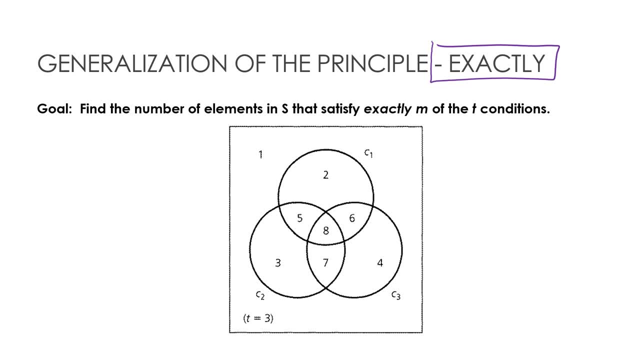 certain number of conditions and obviously in this case I'm looking at three conditions, because I have condition one, condition two, condition three. So that would be my T in this case is that I have three conditions. Say, for instance, I want to find the number of elements where exactly one? 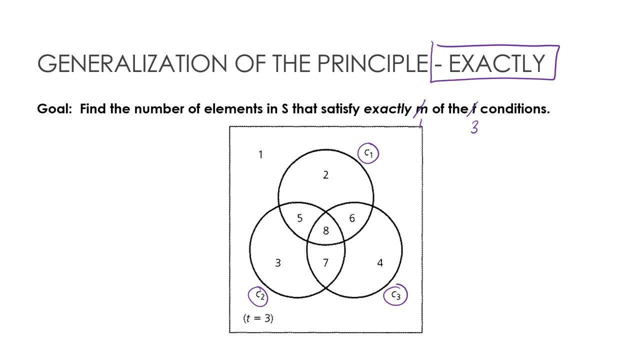 of those conditions are met. Well, in this case, I would want to find this region where only condition two is met, this region where only condition one is met, and this region where only condition three is met. Any of the regions like five, six, eight or seven would be where more than 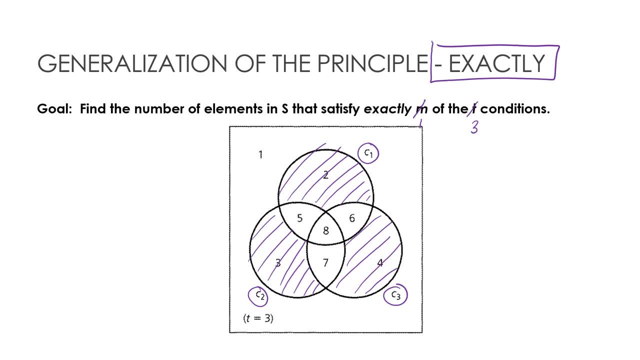 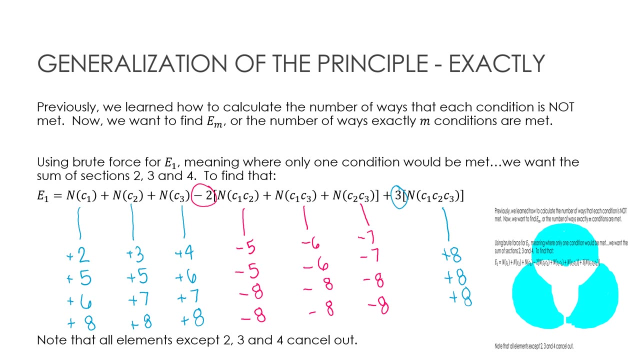 one condition is met, and that's not what I'm looking for at this time. So obviously that would be pretty easy to do if I already had the values on there. but we want to obviously generalize so that we know how would we handle this, no matter what. Again, in our last section we were looking 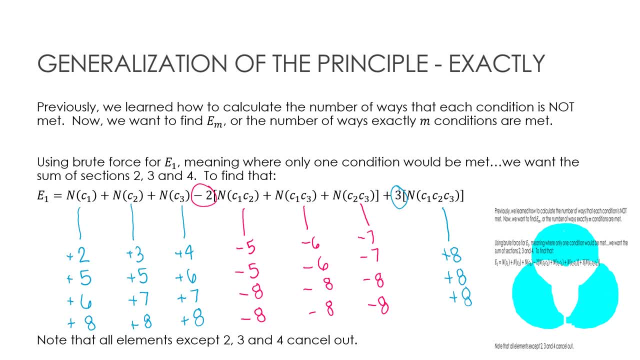 at the number of ways the condition is not met. So in this case, we're going to flip it around just a little bit. and if I were doing this by brute force, and again notice that I've colored in sections two, three and four? Those sections are the ones that I'm looking for, So I'm going to 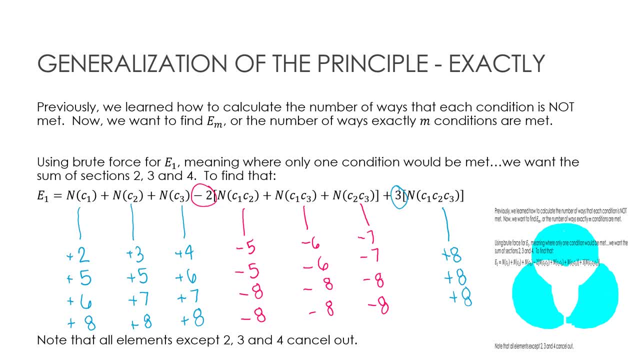 take all of the sections that are the ones that I would want Notice how I'm going to find this and why this works out. I'm going to take all of these, which are where exactly one condition is met and, if you'll notice, for C1, I have just listed the two, five, six and eight that are all within C1,. 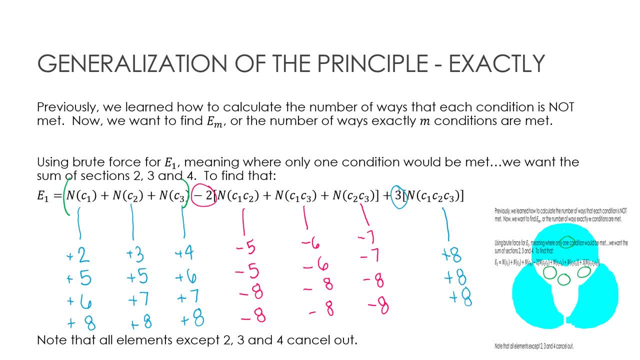 and I repeated that for C2 and C3.. And then I subtracted two of the regions where two conditions were met. So here is where C1 and C2 are both met. Here is where C1 and C3 are both met. Here is where C2 and C3 are both met. 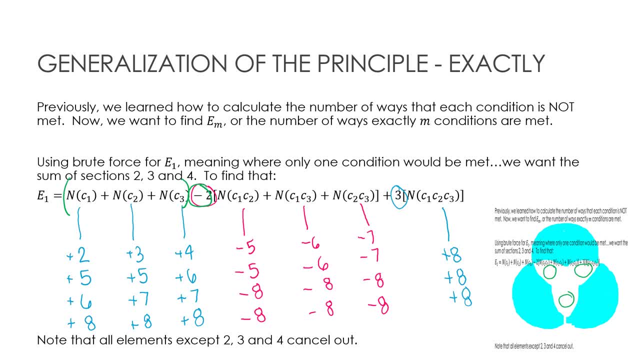 And I've written those in red to note that they are negatives instead. but I've done it twice. so, if you'll recall, why would I do it twice? Because I've counted it here and I've counted it here, So I want to get. 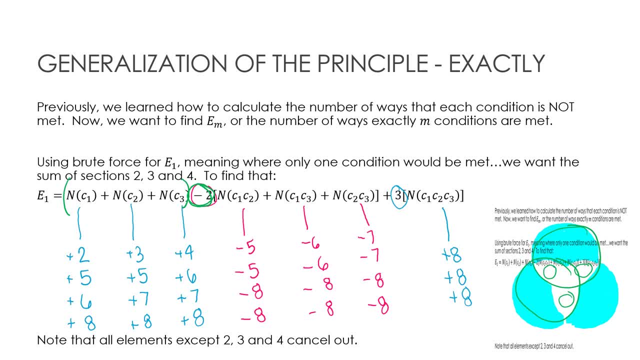 rid of it two times, not just one time this time. And then I continued the same for where all three conditions were met, which is eight, and now I've added it three times. Now, what I want to show you is what happens. I have two- oops, sorry, not two. 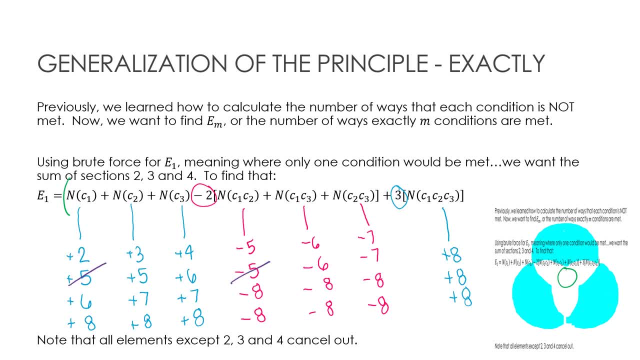 I have five plus five minus five plus five. where's my other? minus five plus six minus six plus six minus six plus seven plus seven minus seven minus seven plus eight plus eight plus eight minus eight minus eight minus eight. 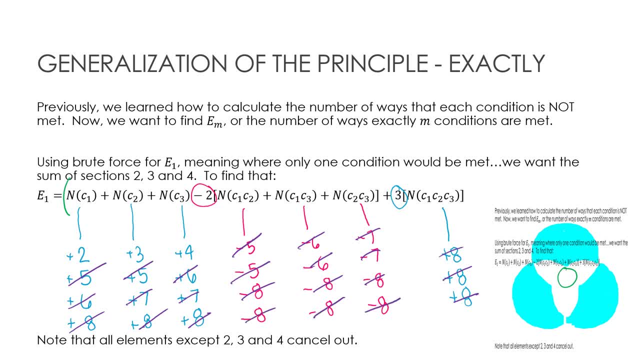 plus eight plus eight plus eight minus eight minus eight minus eight. Notice, all I have left is two, three, four. So really I've gone about it in sort of a long way, but as usual, we're not going to go through this much work. 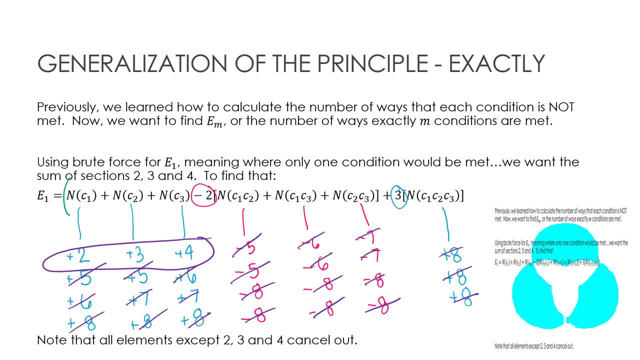 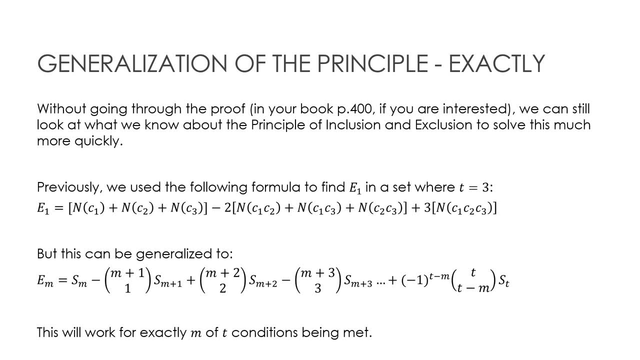 We're going to generalize to make it easier for ourselves to do this. Now, for those of you who are interested, you are welcome to look at the proof of the exactly generalization of the principle in your textbook, Page 400.. But really what we're going to do is look at the principle of inclusion and exclusion and how we can solve this. 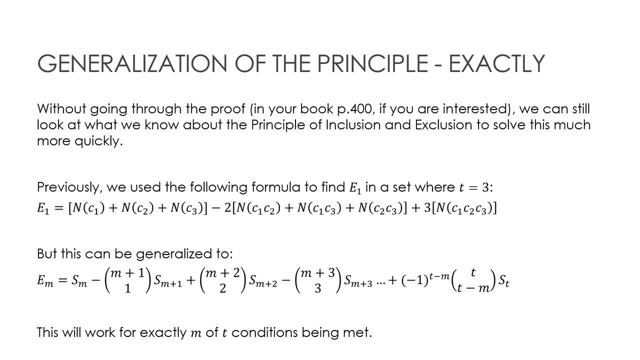 So we really want to generalize And keep in mind we're looking at T conditions And we're looking for exactly M of those met. Now here's what we did just a moment ago on the other side, and this worked where T was equal to three. 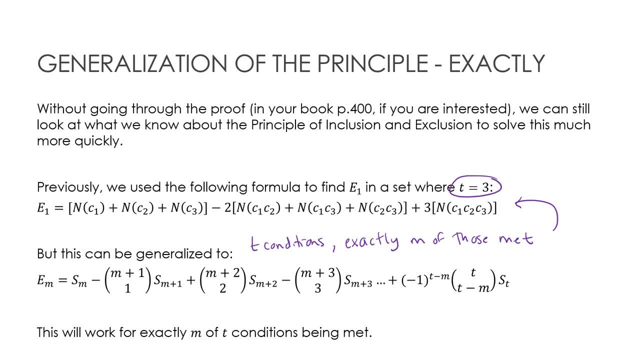 But that's not a generalization, because we don't want to have to memorize it. We don't want to generalize anything, We just want the formula that's going to work all of the time. And I do want to point out, before we look at the generalized formula, that I'm looking at E1, which means this is exactly one condition is met. 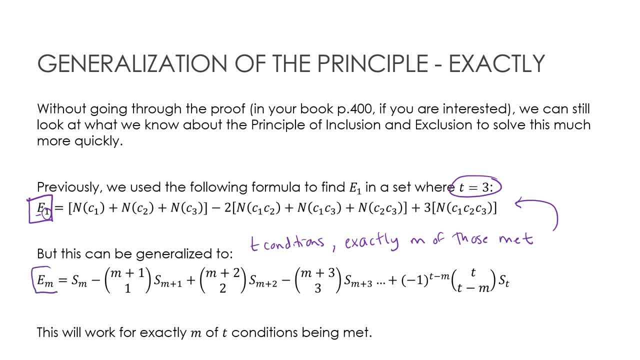 So that's what we worked on on the other page. So here's the generalization: E, M, which means exactly M of those conditions are met. We're going to start with M, which means just the set of exactly those being met, just like we did before. 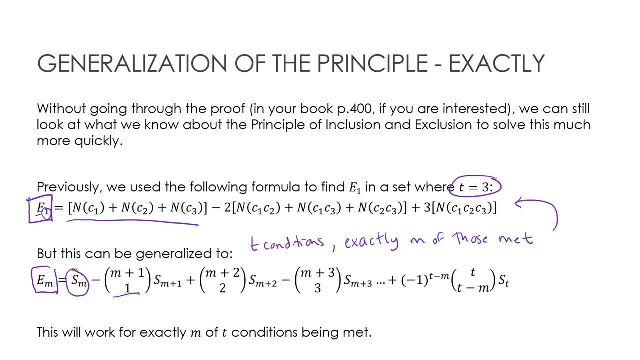 Then we're going to use that binomial coefficient and that's going to be the magic that gives us the two And the three, et cetera, so that we don't have to calculate those ourselves. So here's our formula that says: you're going to now take 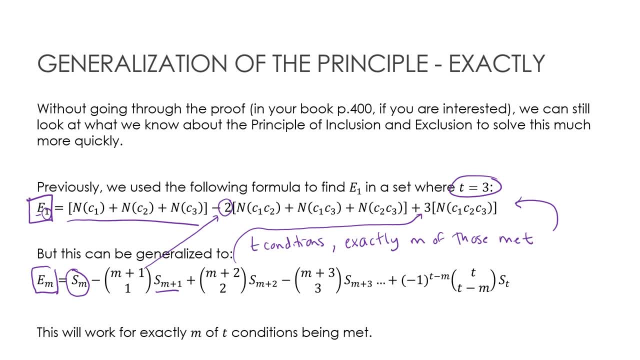 How many times two of the conditions are met. If you're looking at M equals one, then three of the conditions are met, except et cetera, all the way up to T, which is how many total conditions that you have. 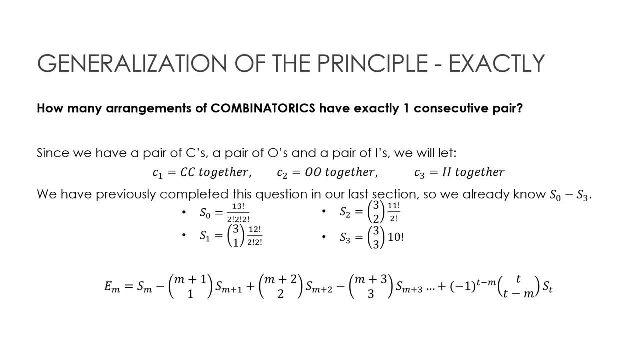 So let's take a look at this in action. Here's a question that should look familiar, and you'll note that I've just changed it a little bit. We previously looked at combinatorics and we were looking at how many don't have any pairs together. 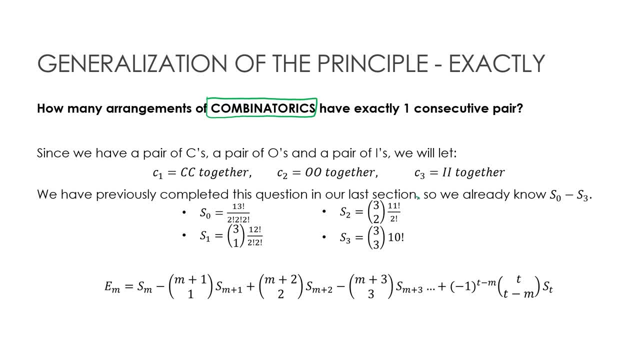 And so when we did that, we came up with our values, All of these values. So if you didn't watch the last video, make sure you go back and watch that video, because we talked about where all of those came from, But really we just said, hey, there's 13 letters. 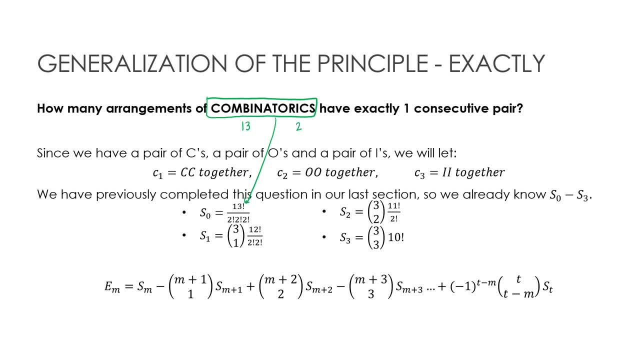 And we've got A set of two O's, A set of two C's And a set of two I's, And then we continued looking at that pattern, for if one condition, two conditions, three conditions were met. So I don't want to waste time going through that again. 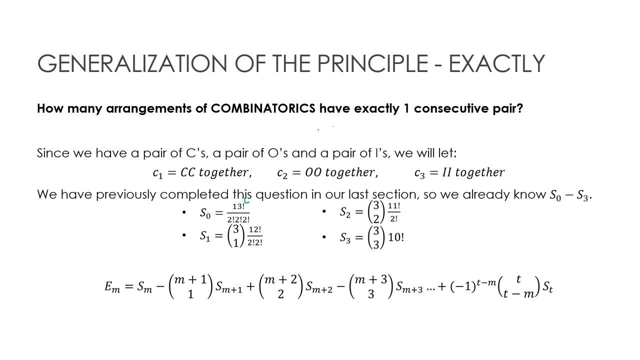 Just go back to that first video. So again, here's what we have so far, And then here's this new formula that we just came up with. So let's take a look at how I would go about this. So if I want to know exactly one consecutive pair, then I'm finding E, sub one. 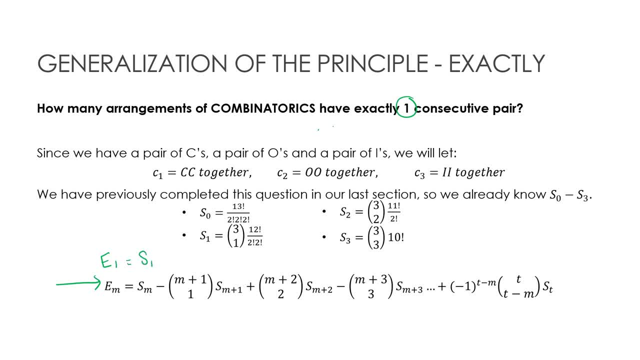 Which means I'm going to do S sub one first, Because M is equal to one and T is equal to three, Because we have three total pairs. There's three conditions. So S sub one minus, This would be one plus one or two. 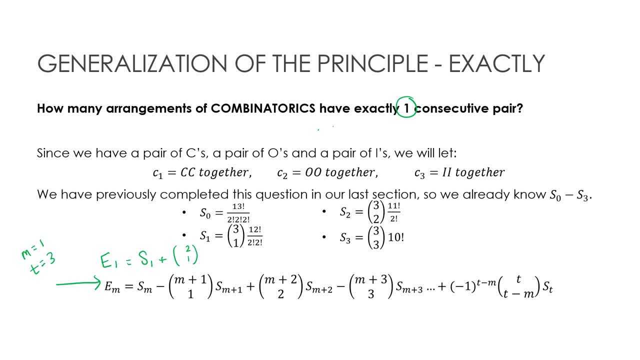 Choose one Of S sub two. Oops, that was a minus, And then this one is a plus, And then it's going to be one plus two or three. choose two S, three, And of course that's where we can stop, because three is T. 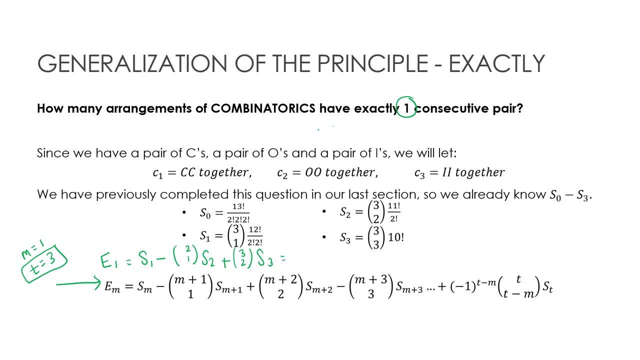 And that's where we stop. So, really, all I'm going to do, then, is sub in what I know: Three choose one. Twelve factorial Two. factorial two. factorial Minus Two choose one, And then S two Is three choose two. 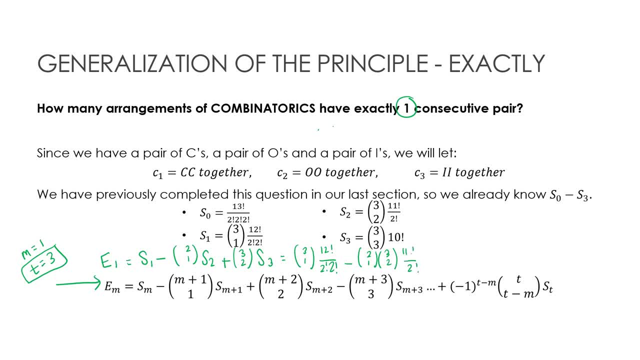 Eleven factorial over two factorial Plus Three choose two, S three And S three was three choose three, Ten factorial. So we can see that that would be my solution And again, It's really not necessary for you to go ahead and multiply everything out. 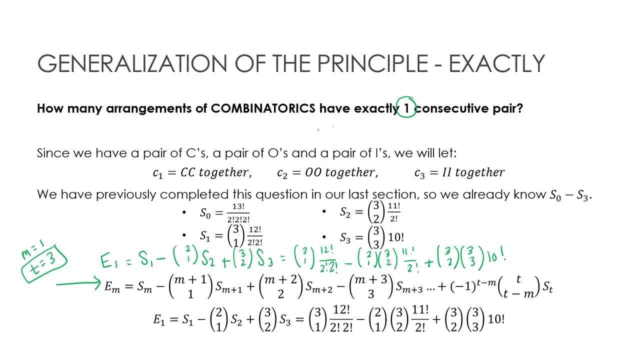 It's kind of a waste because, yes, you can find the exact solution. So only if it says find the exact solution would I go through the trouble of actually working it out. Mostly I'm just worried about: can you come up with the correct expression that comes to the correct solution? 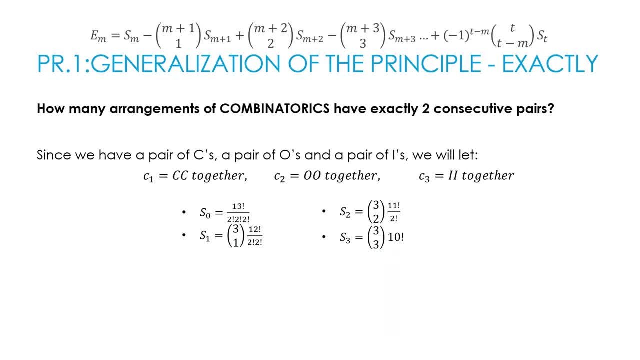 First practice on your own. I wanted you to do basically the exact same question, Except for notice. now we're looking at exactly two consecutive pairs. Keep in mind T is still three, because I still have three pairs that are possible. M, in this case, would be two. 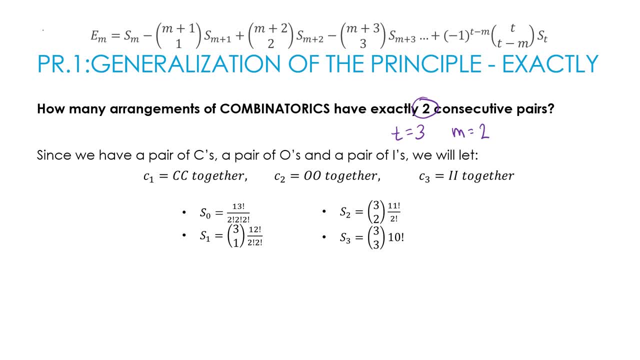 So it's going to be just a little bit different, But I have given you that formula because I don't expect you to have it memorized at this point. So go ahead and complete this question And, when you're ready, press play to see how you did. 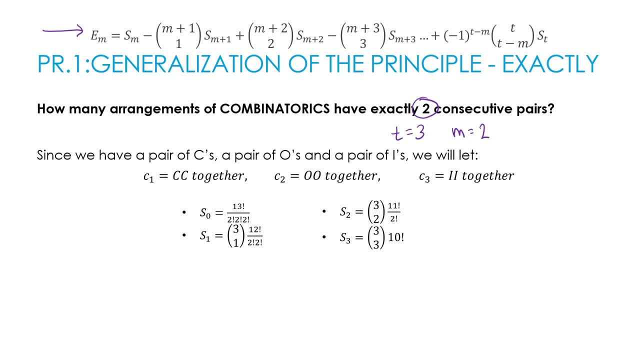 So again, in this case we are looking at: M equals two, So I'm going to find E2, which means I'm starting with S2.. And I'm really only going up to S3, because that's the highest number. So for my first one it's just S2.. 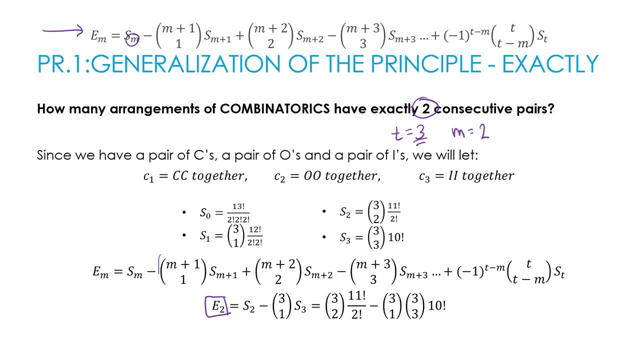 For my second one it's two plus one. So really I'm only using up to this point in this solution, So I'm taking two plus one, which is three, Choose one And then whatever S3 is, And S3, again we already had- was three. 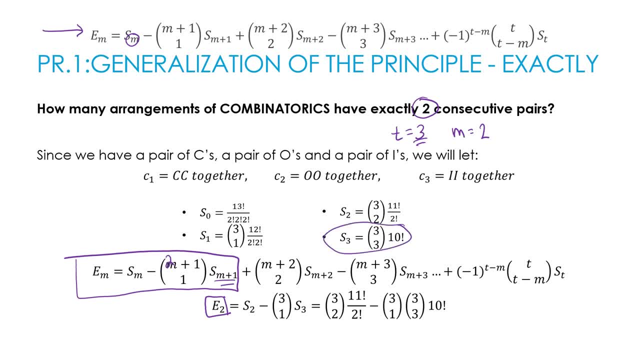 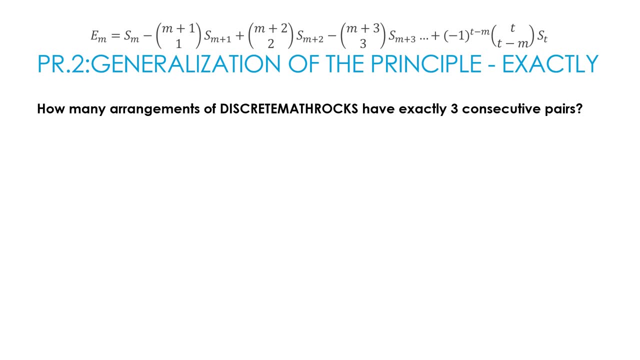 Choose three, Ten factorial. So that's all we have to do. Here is my final solution. So here's a question that we haven't done before. This one's going to be a little bit harder because we haven't found S0, S1,, S2, etc. 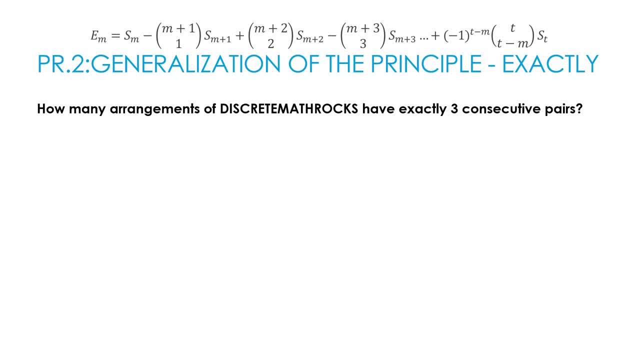 Or however many S's you need to find. So this one will take you a little longer, But again, I encourage you to please try this one on your own. Don't just wait for me to go through it. So I'm going to give you a minute. 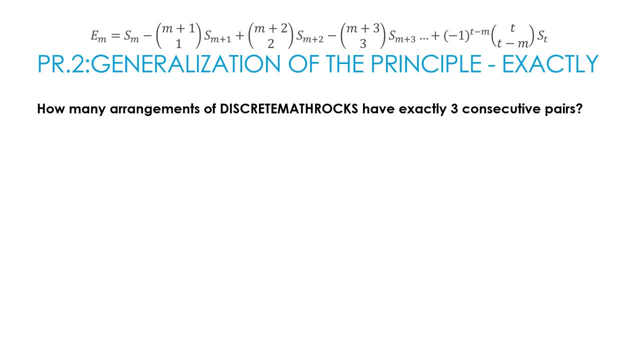 I want you first to find what are the conditions, which means take a look at discrete math- rocks, which is our word- And find out how many pairs we have, because we're looking at consecutive pairs. So find out how many pairs we have. 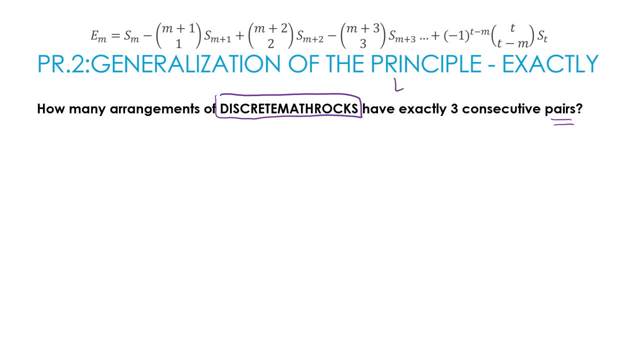 And that's going to be T, And then M is obviously going to be three, because we're looking at three consecutive pairs. So find all of those values first and then simply plug them into this formula. When you're ready to go, press play to see how you did. 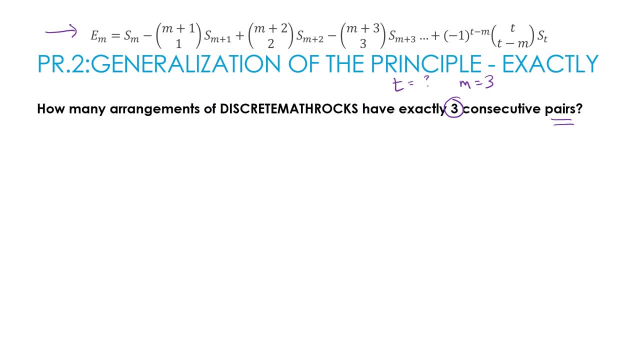 So again, where would I start? I would look at the word discrete math rocks. So I've got a D here, but I don't have another D. I have an I, but not another I. I do have an S with another S. 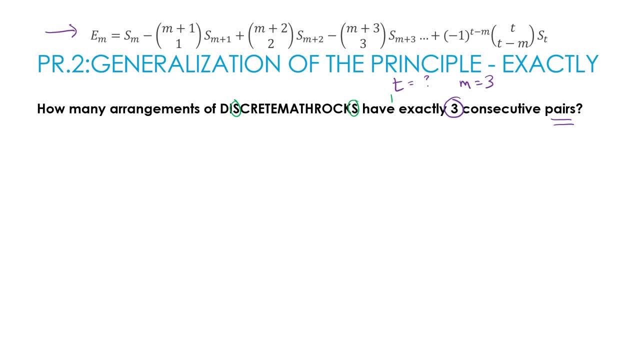 So I'm just going to keep a tally. I have a C and another C. I've got an R and another R. I've got an E and another E M. I don't have another one of. Oops, I almost forgot my T. 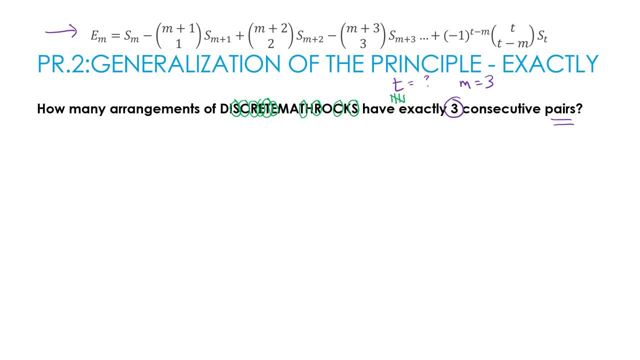 T. I have a pair M. I do not have a pair A. I do not have a pair H. I do not have a pair O. Okay, I don't have any more pairs. So it looks to me that T is equal to 5,. 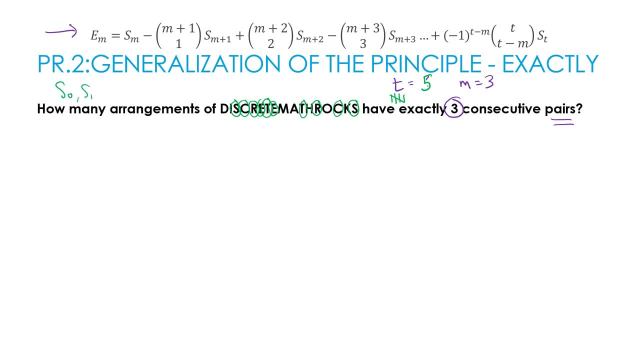 which means I need to find S0, S1, S2,, S3,, S4, S5.. So the conditions would be that the S's are together, or the C's are together, or the, et cetera, et cetera. 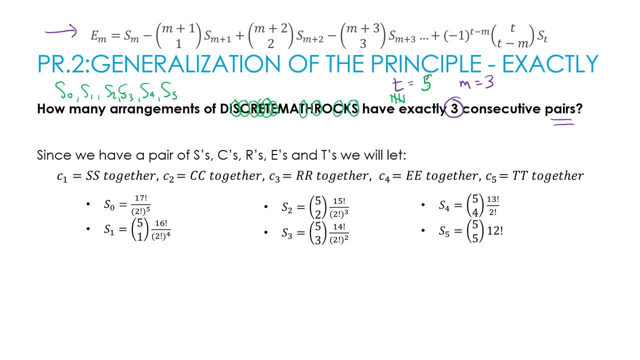 You get the idea. So that's the first thing we want to do is to find the S's, the C's, the R's, the E's and T's. That's the five conditions, And we're going to go about it the same way we did in our combinatorics. example. 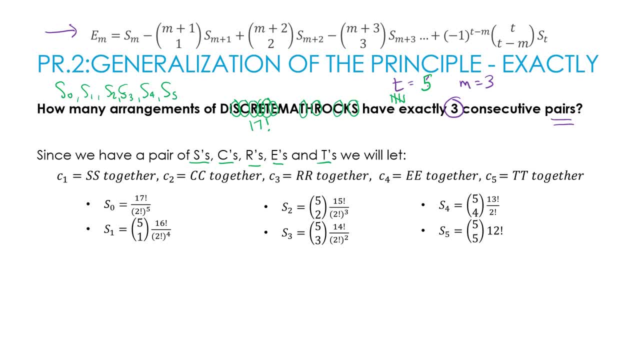 I have 17 total letters, That's 17 factorial. I've got 5 sets of 2.. So 2 factorial 5 times. So notice, I just wrote it 2 factorial to the 5th. Then when I say one condition is met, 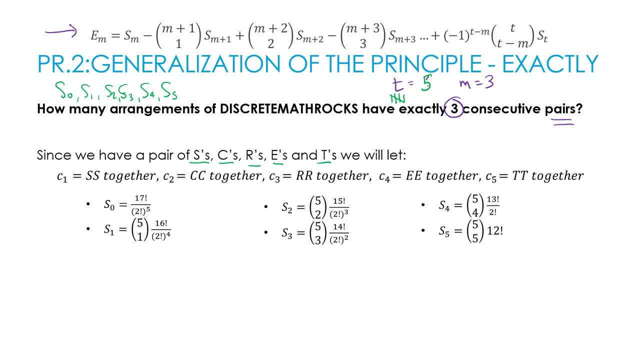 actually I'm saying: let's pretend that I've created a letter or I created a word where two S's are together, So D-I-S-S, and then everything else is the same until I get to the end and I just drop the S off. the end would be an example. 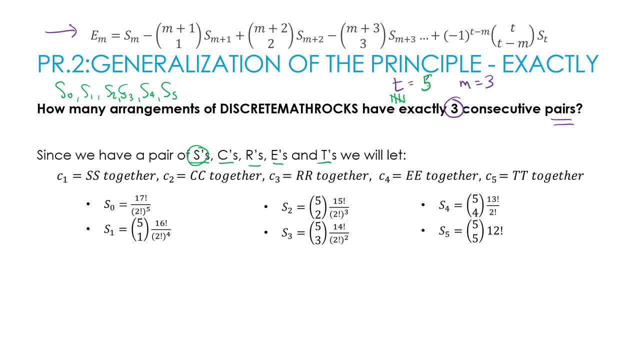 where my two S's were together, which means if I've taken two S's and plugged them together, that's just one letter. So now I have 16 total letters and I only have 4 other pairs That could or could not be together. essentially, 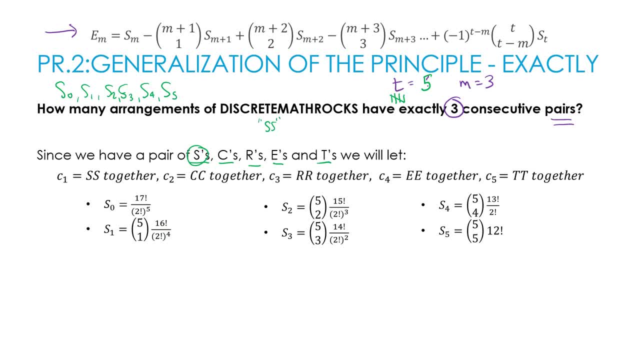 And then, where does this 5 choose 1 come from? Because there are five conditions and I'm choosing one of them to be met, And I continue that for S2.. So notice, this is decreasing by one. This is decreasing by one. 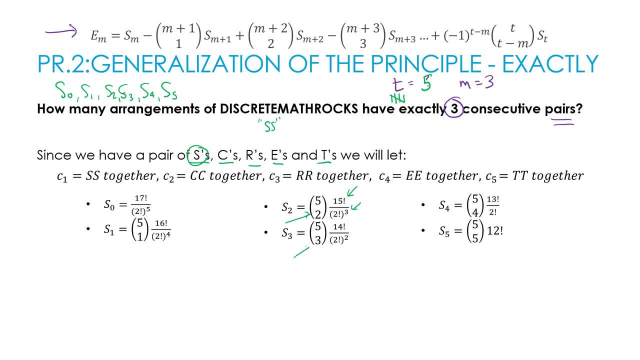 This is 5 choose 2, because it's two conditions: 5 choose 3, same pattern. These are decreasing, et cetera, et cetera. So that's where those values come from, And now all I have to do is take this and plug in my values. 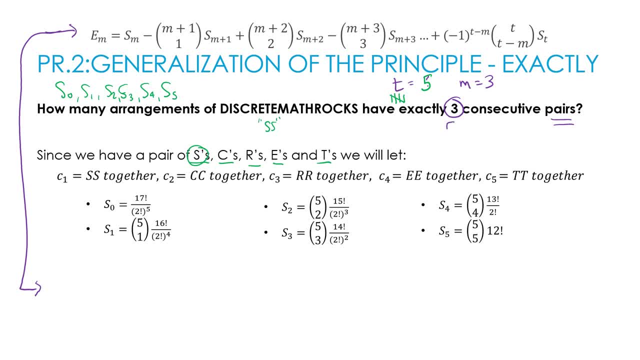 So I'm looking for E3,, which means this is going to be a 3.. This is going to be a 3.. This is going to be a 3 plus 1,, which is 4.. This is going to be a 3 plus 2,, which is 5.. 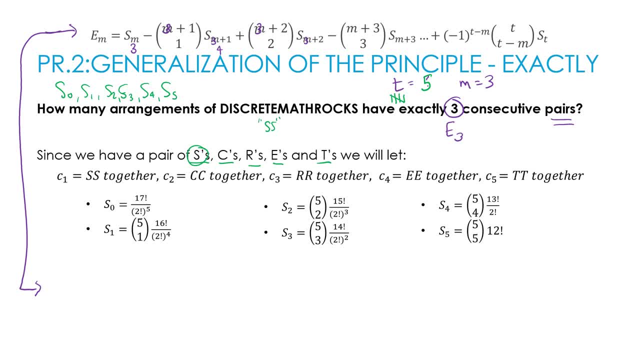 This is going to be a 3 plus 2, which is 5.. And I'm obviously going to stop there Because there are only five. So notice, that's exactly what I'm doing here: 4 choose 1,. 5 choose 2 of S3, S4, S5. 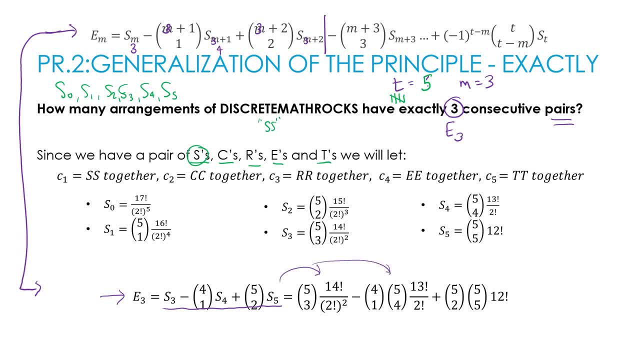 And then I'm simply just subbing in what I know for S2, or, sorry, S3,, S4, and S5. And again, leave your solution just like this. There's no reason for you to multiply everything out and add and subtract, et cetera. 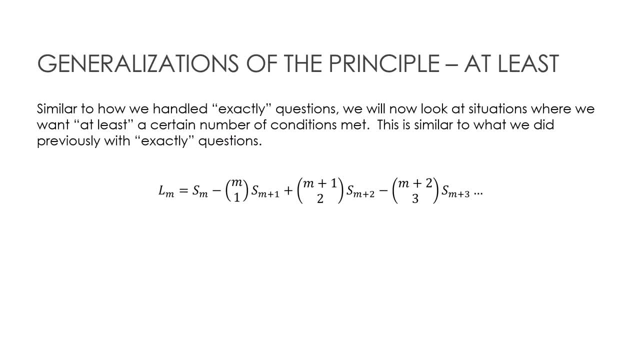 So this brings us to our, at least, questions, And at least, obviously, is going to be just a little bit different, because instead of exactly, we're saying exactly that or more, And the only difference really that we're looking at is when we were looking at exactly some number. 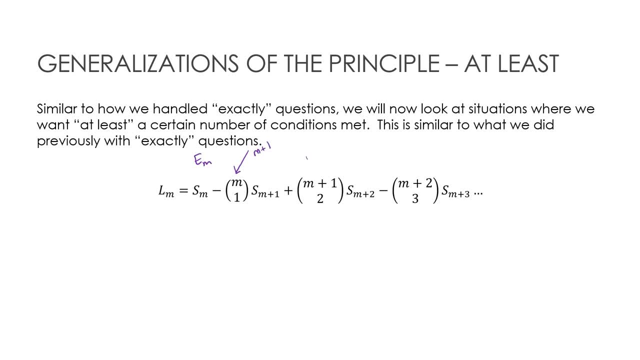 this top value was M plus 1, and it continued to increase M plus 2.. Now, if you'll notice, we're just starting at M, going to M plus 1, M plus 2.. But really everything else is the same. 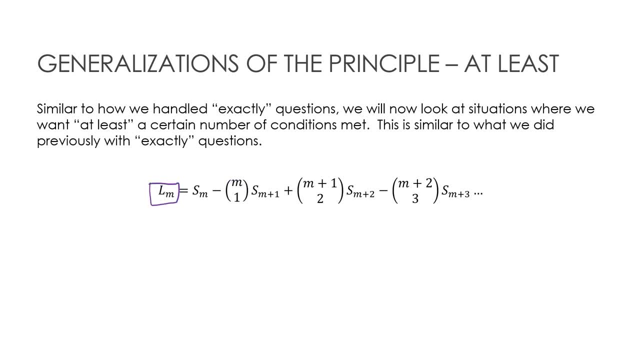 And, in addition, keep in mind, now you're going to see the L, So keep those straight, so that when I ask you a question I might not say at least, or exactly. I might just give you this at the beginning and expect you to know that that means at least. 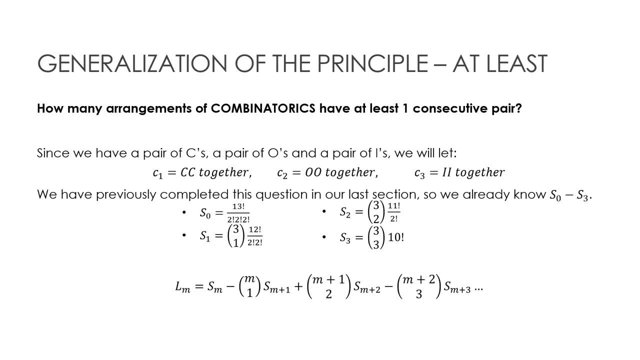 We're going to start with an easy one. Easy because we've already gone through and found all of these values for combinatorics And in this case we're saying at least one consecutive pair. So previously we found no consecutive pairs and we found exactly one. 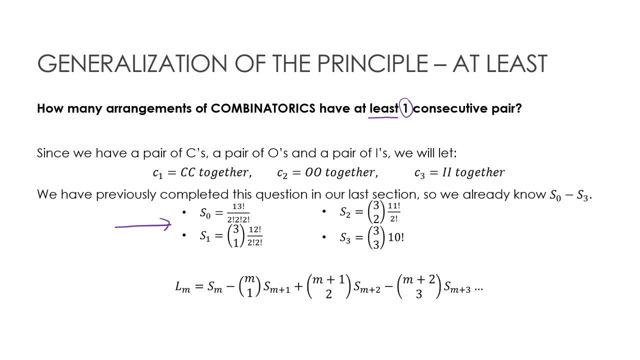 Now we're saying at least one, So one consecutive pair, two or three. How do we do it Again? we're just going to plug values into this formula. So T is still 3 because we have three conditions or three pairs. 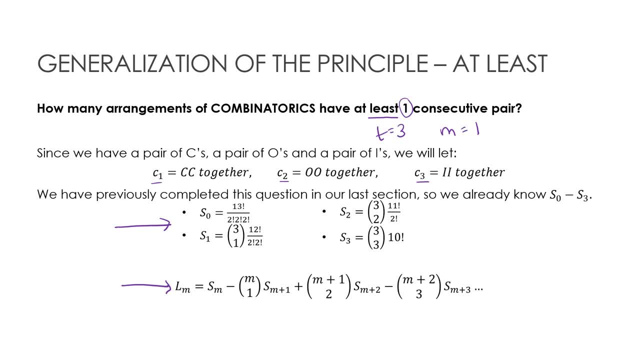 And we're saying one or more is met. This is going to be a 1.. This is a 1.. This is a 1.. This is a 1 plus 1 or 2.. This is a 1 plus 1 or 2.. 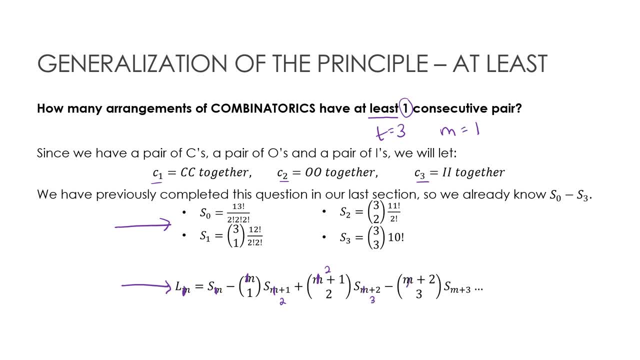 You get the idea. Really, all we're doing is coming up with the values. Well, actually, this one I don't even need to do because I don't have that many, So all I'm going to do is plug in values from up here. 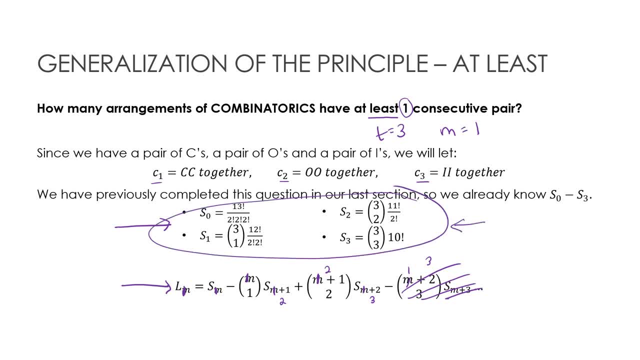 which means this is the hardest part, people, because if you have that formula in front of you, you're just plugging things in. So let's take a look. S1,, which is 3 choose 1, 12 factorial over 2 factorial, 2 factorial. 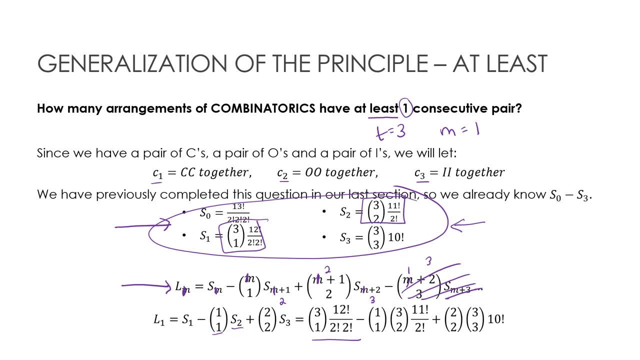 1 choose 1 of S2, which is 3 choose 2, 11 factorial over 2 factorial, And then 2 choose 2 of S3, so 2 choose 2 of 3 choose 3, 10 factorial. 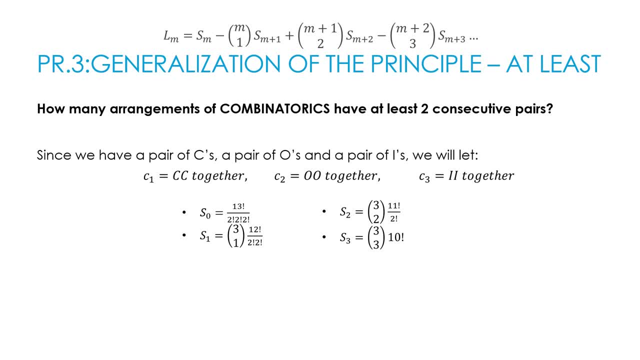 That's the final solution. Again, here's a fairly straightforward one for you to try yourself. We already have all of our different possibilities laid out. That makes it super-duper easy. So use that formula to come up with at least 2,. 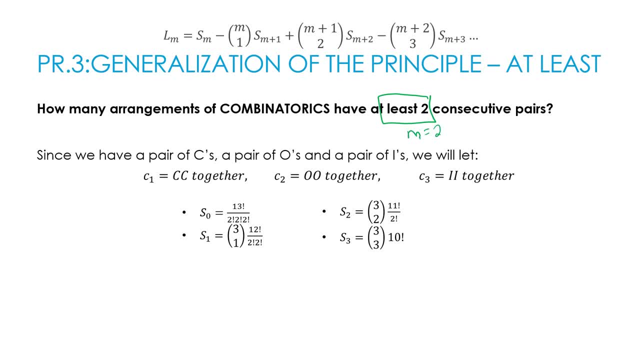 which means M is going to be 2.. When you're ready, press play to see how you did So again. I've just recopied it here, So we know what we're dealing with. I'm starting with: M is 2.. 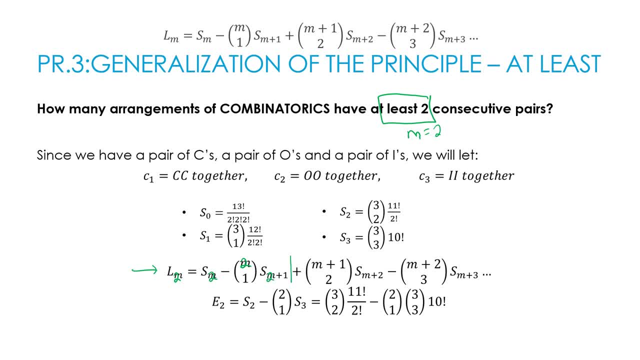 And obviously I'm going to stop right there, because 2 plus 1 is 3.. So that's all I have to do is: S2 minus 2, choose 1 over S. sorry, 2, choose 1 times S3.. 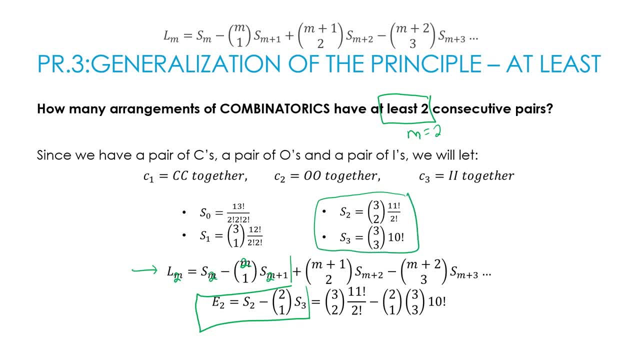 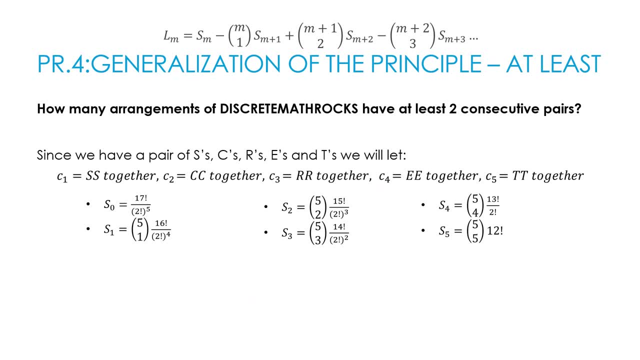 And again I'm just finding those values here which we already determined. Just one more easier example, Because today, just a bit earlier, we already went through and found this together And honestly, I think that is the hardest part, But again, it's just an acquired skill. 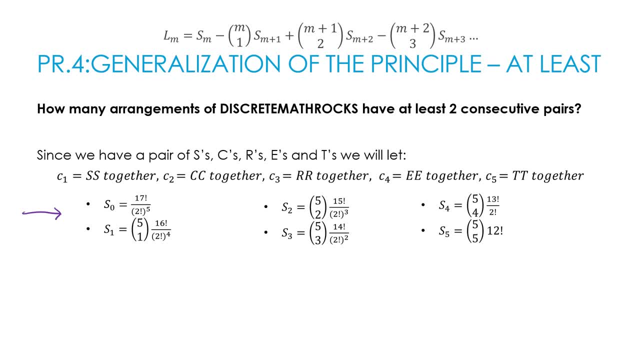 The more you practice, the better you get at it. Here we're looking for at least 2 consecutive pairs, So M is going to be 2.. And we're going to continue until we have M of 5.. So really, I'm going to be using all of these. 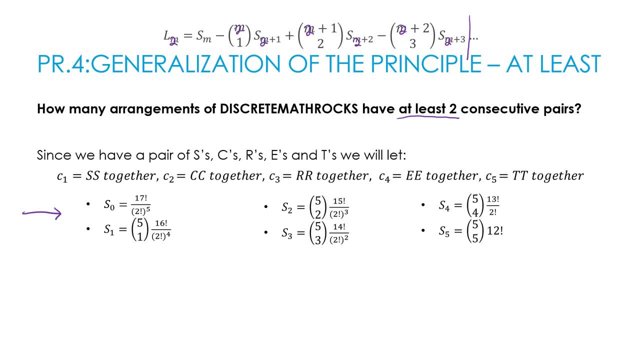 So, basically, I just want you to write out the expression And, when you are ready, press play to see how you did So. again, I'm looking for L2.. That's important to put in the front, because that signifies that we're looking for at least 2.. 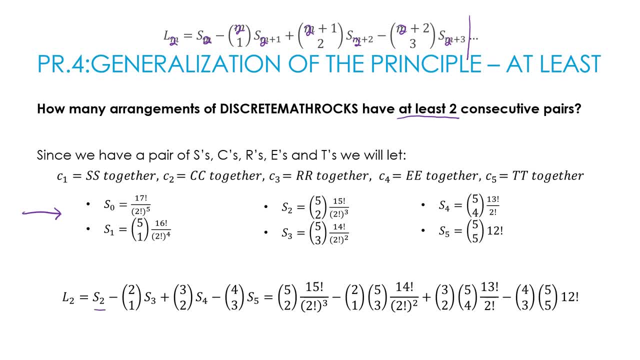 We start with S2.. And then we have M over 1, S3.. M plus 1,, which is 2 plus 1, or 3. M plus 2,, which is 2 plus 2. Or 4.. 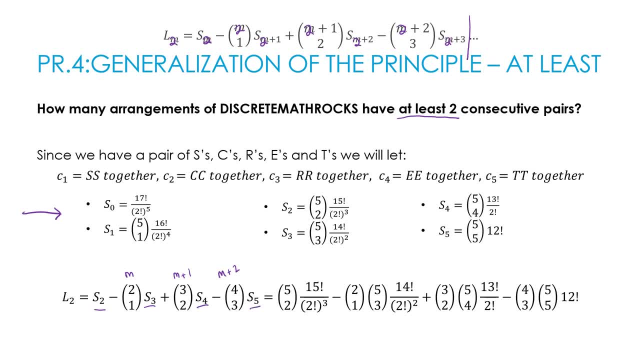 And again. then I'm just going to replace all of those S's with the values that I've already found. So here is my final solution, And again I'll say: leave your answer just like that. So for your last question I wanted to give you one. 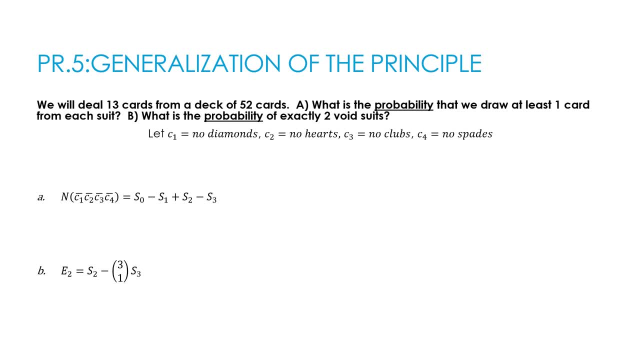 that would make you think a little bit more, And I have given you a couple of hints for both A and for B, But obviously this is a two-part question. Again, my suggestion is: first try to figure out what S0 is. 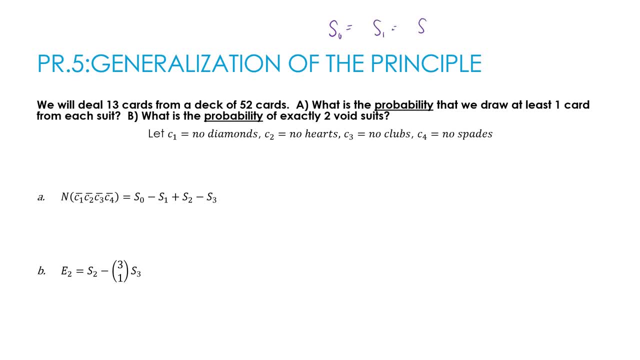 S1, S2, S3, S4.. Now why did I stop at 4? Because there's going to be four conditions. Why are there four conditions? Because we're talking about suits of cards And there are four suits. 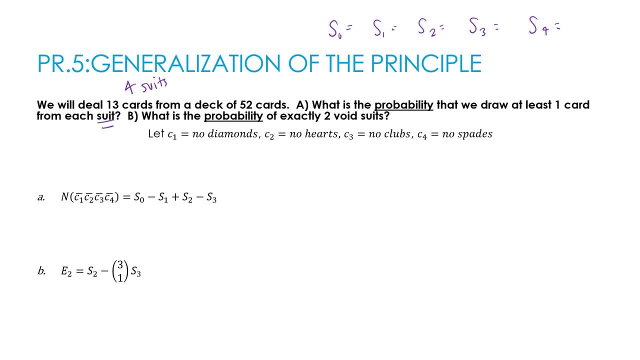 Hopefully we all know that. If you've ever done anything with probability, you should know that there are four suits in a deck of cards, There are 13 from each suit, et cetera, et cetera. So you might get a little bit confused at how I set up A. 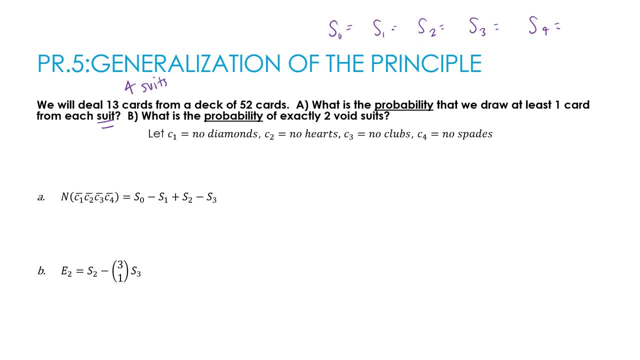 But really it's the same as me. Well, I'm going to wait to go through that. So I've given you a couple of hints for A and for B, But again, start by finding these values Because, remember, that's generally the hardest part. 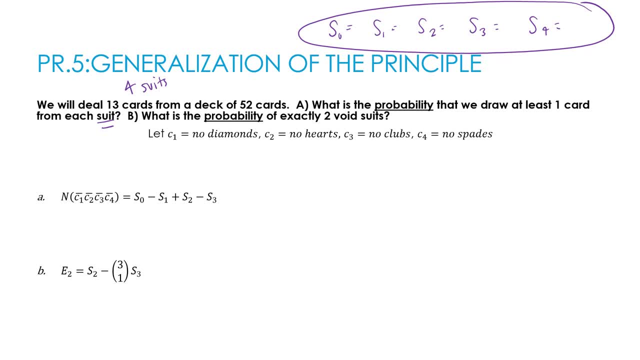 Then, when you're ready, go ahead and compute the values that I've laid out for A and B, But also keep in mind the fact that we're looking at probability. Now we haven't talked about probability yet, but it's going to require an extra step. 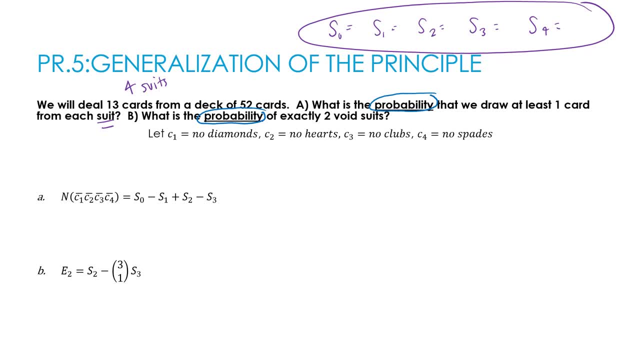 So, when you've had a chance to really think through this- and it's okay to pause it for more than a couple of minutes- really try this question first. When you are ready, press play to see how you did. So, again, the first thing I want to do: 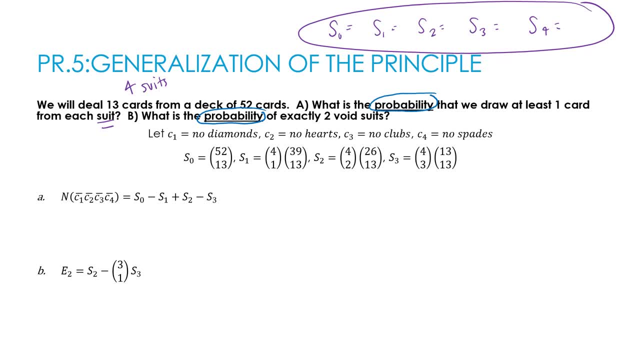 is come up with my S0.. S0, S1,, S2,, S3, etc. And notice, I stopped at S4 because each time there are- in this case there are 52 cards and there are 13 of one suit. 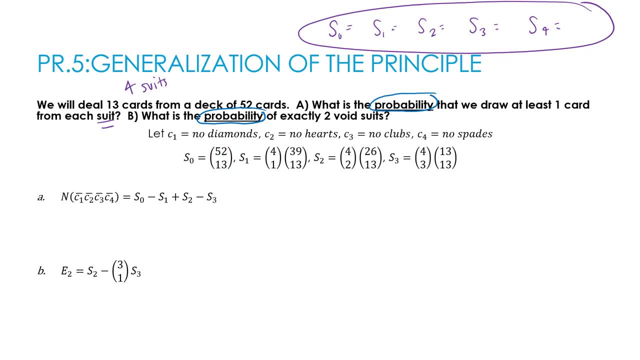 So then my next one was: hey, there's four conditions And really in front of this is a 4-choose-0, which is just one. So it's okay not to put 4-choose-0.. But this is 4-choose-1.. 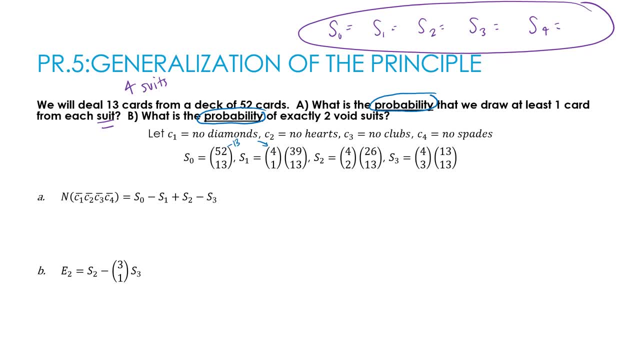 And then notice I've just taken 52 minus 13,, because again I'm taking away the 13,, say diamonds etc. And saying now what's the chances or how many options are there if two conditions are met? 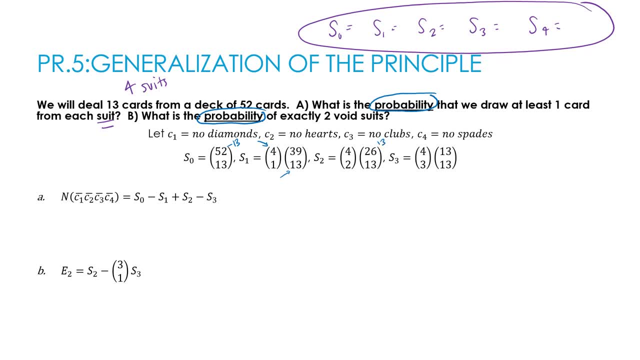 And again I've subtracted 13. And so if I did an S4, it would be 4-choose-4 of 0-choose-13,, which would be silly, which is why I didn't include it. So now let's talk about. 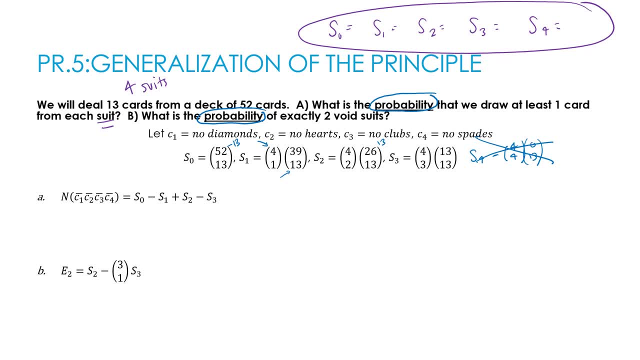 how to solve for these questions. So for the first one, again you might be confused and say: well, why did you choose this? in order to compute? Well, this in order to compute is essentially saying: and notice that my conditions were. 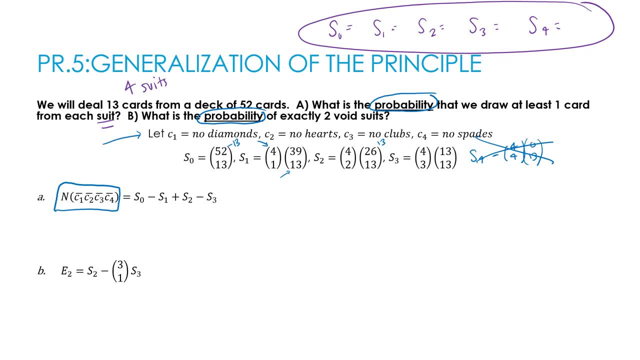 no diamonds, no hearts, no clubs, no spades. So what I'm looking for is that I draw at least one card from each suit, and so that's the same as me saying I didn't get none of each suit, because that would mean I got at least one. 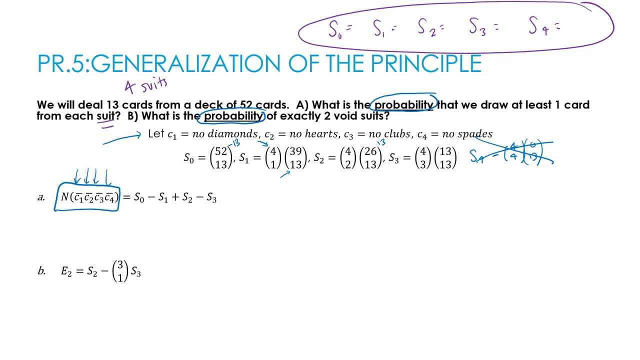 from each suit. The other way I could go about this- and I'm telling you this is going to give you the exact same solution- is: if I found L1, I'm sorry if I found not L1,, if I found exactly zero. 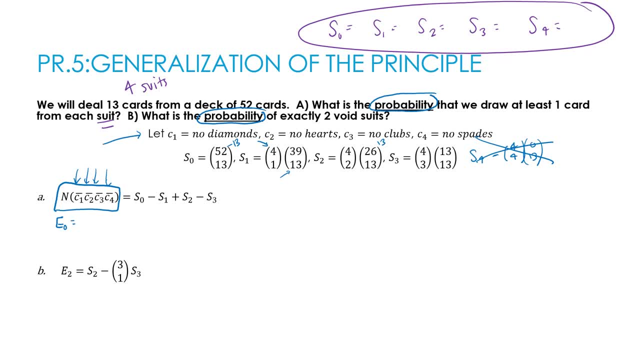 Now exactly zero, because again we're saying at least one card from each suit, but my conditions say no, no, no. So I'm saying let's find the number of possibilities of getting exactly zero conditions met. None of these conditions are going to be met. 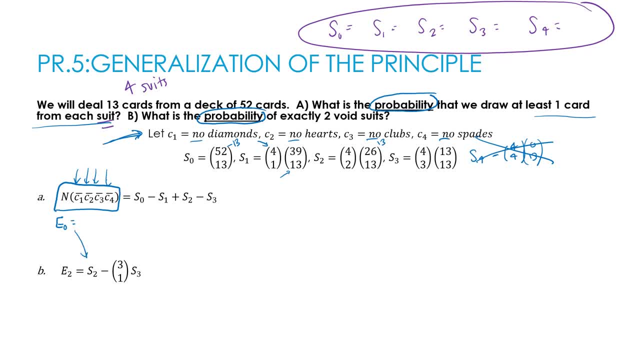 And so I'm going to do it like I do it here, where I start with S0, and then I have minus three, choose one, S1,, et cetera, et cetera. Now, I'm sorry, not three, choose one. 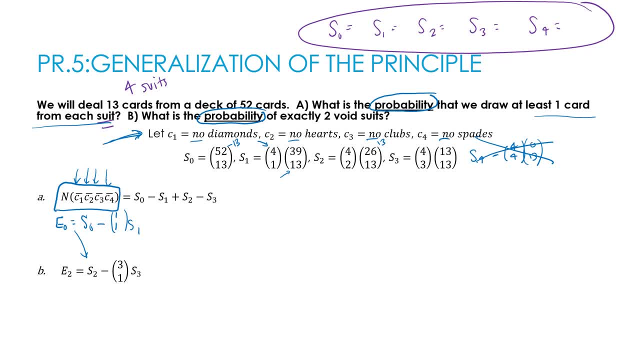 one choose one. Now why does that matter? Because one choose one is one, and that's just going to give me the S1.. And then I'm going to add two- choose two- S2, and subtract three- choose three- S3. 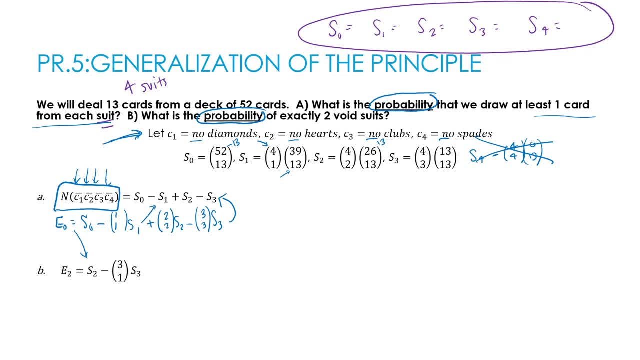 And, if you'll notice, that's exactly what I have here. So now we need to look at the fact that we're looking at a probability, and probability is something we haven't done yet. So the only thing different- and let me get rid of all of this: chicken scratch. 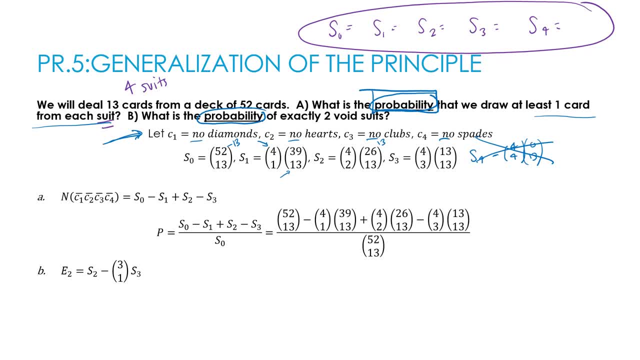 The only thing different is saying: put the number of possibilities, which is this guy which is the same as me, saying exactly zero, which we just talked about, divided by the sample size, which is the universe. So notice, my denominator is just 52, choose 13.. 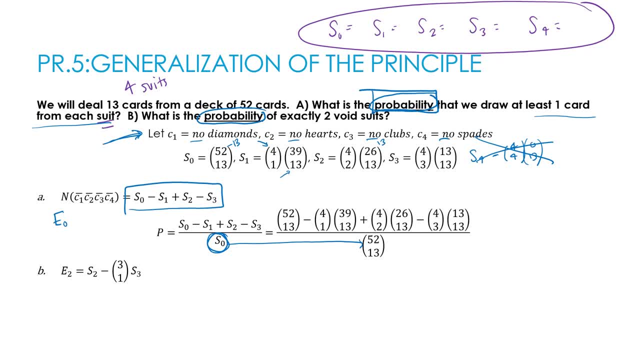 For the second question again, two void suits means essentially that exactly two conditions are met, which means exactly two conditions are not met, et cetera. You get the idea: Exactly two conditions are met. So my numerator is going to be this guy. 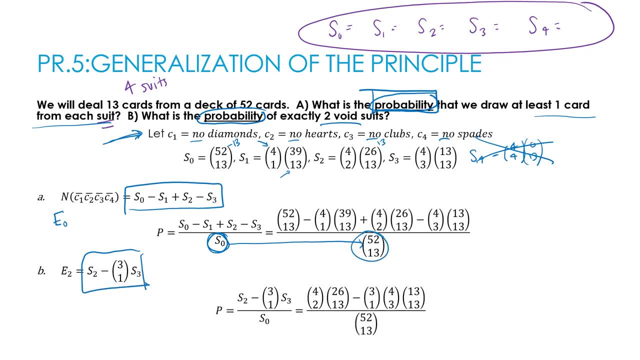 My denominator- yep, still this guy. So I'm taking the probability- is S2 minus three. choose one S3 over S0, and this is the value that I come up with. So don't be hard on yourself if those were difficult for you. 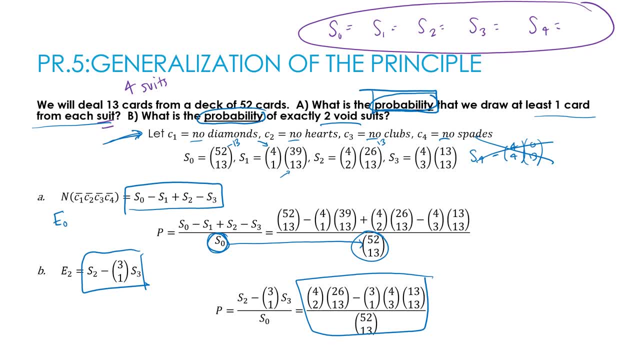 They were meant to be difficult for you. Stay tuned. In our next video we're going to be looking at derangements.